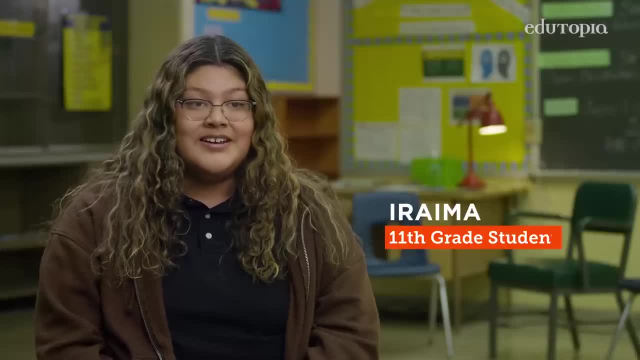 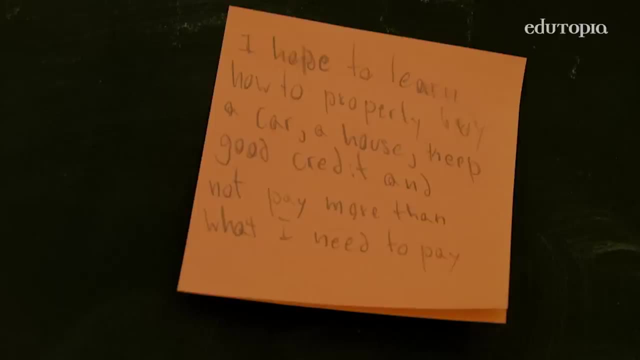 When we first started learning about financial literacy, I was definitely scared because I was like whoa, I'm growing up. But it's pretty beneficial, especially if you're trying to get a debit card first job, eventually building credit. 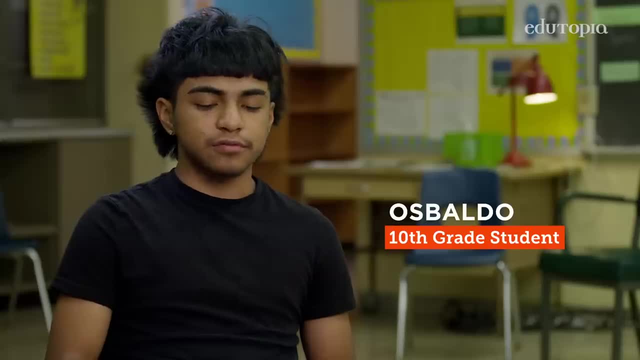 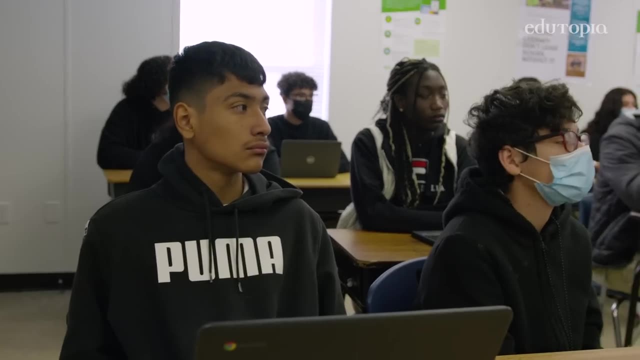 I started working at the age of 14, so I pay some bills with my parents whenever they need help. The class has helped me learn like what I should look at when I get my check. I cover a myriad of topics: investing, depository institutions, debt management. 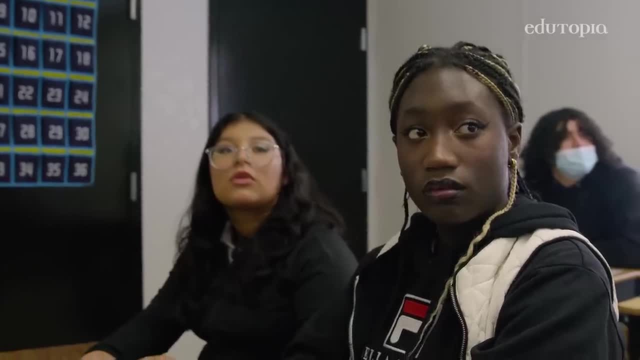 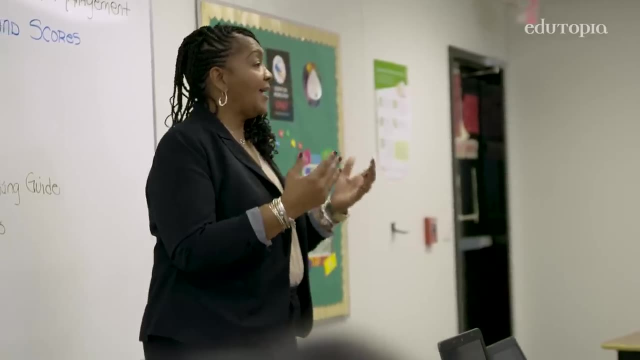 So today we're going to be talking about managing your money. This is called the 20-bean game. The beans will represent your salary And you're going to have to decide where I am going to spend this money. So you're going to be adulting for a minute. 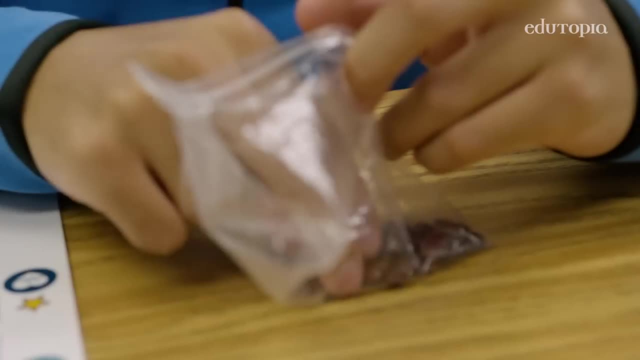 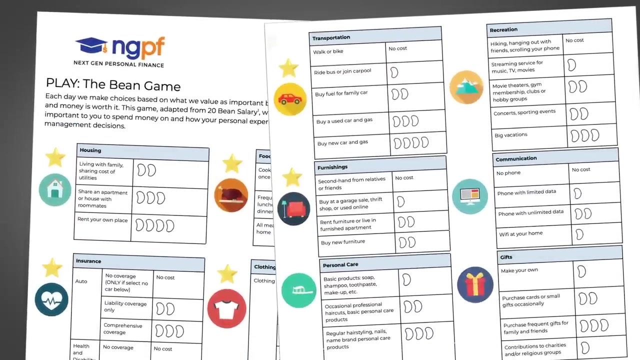 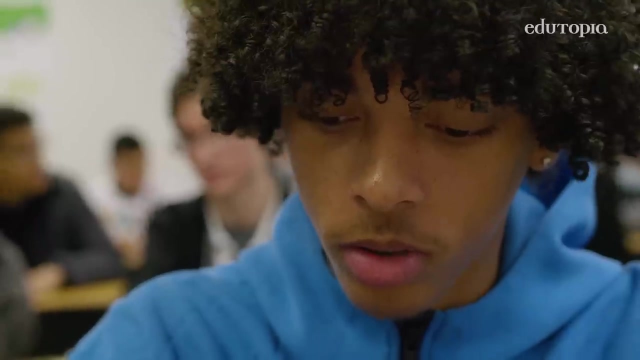 Students were given two sheets where they had to allocate beans to certain categories, six of which were mandatory, such as housing, clothing, food. Each category has a couple of options. If you want to eat at home, it's one bean. If you want to go out all the time, it's three beans. 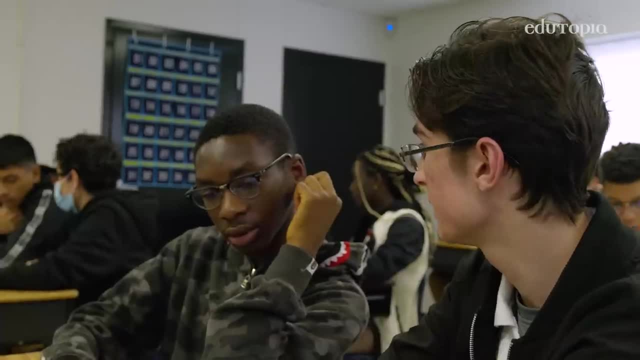 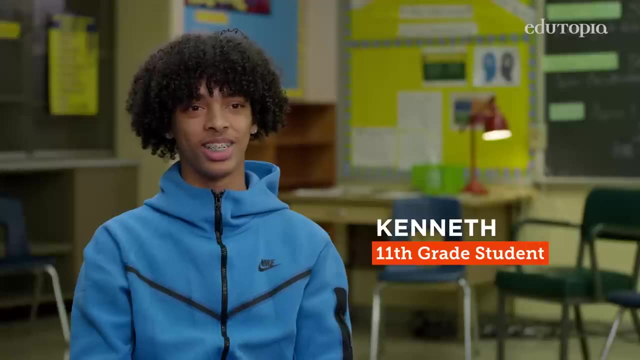 Do we want like our own house? Do we want to share with our family? Oh sure. So we're going cheapo on that. You're not going to be using beans, obviously, Like you're going to be using money, but it's showing you how to like budget your. 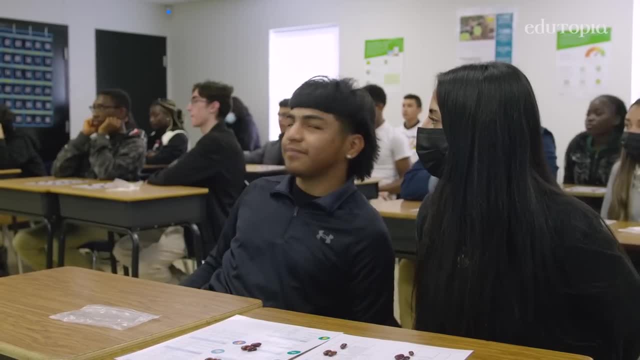 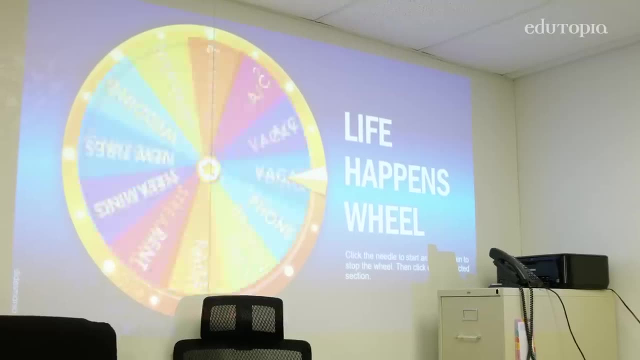 money. Okay, Time's up. We're now getting ready to start round two. I have a spin wheel here, So basically the wheel will spin and then, like something would happen, Tell me when to stop. Stop- Stop. Your microwave broke and you need to replace it. 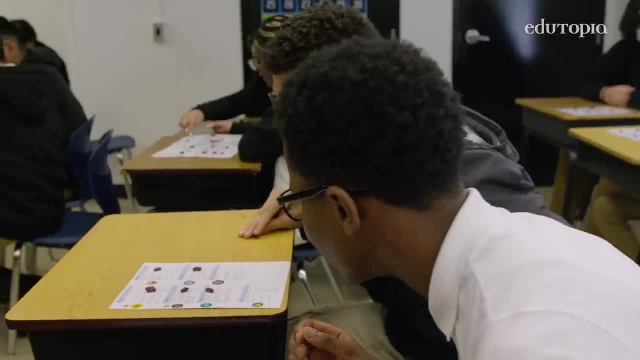 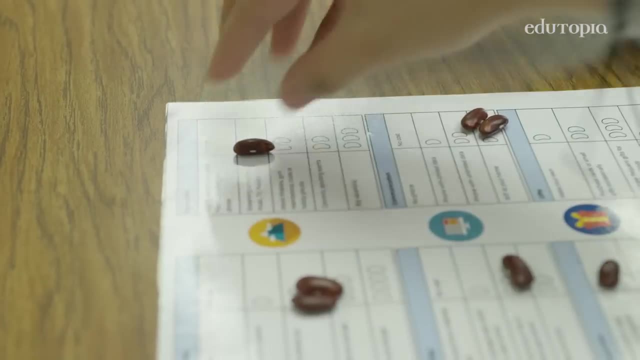 Take off one bean. What Hold on From anywhere. You have to decide where to take a bean. Yeah, Make sure that your star categories are still covered. Take that out. Bye, babe. Okay, My wheel is going around again. 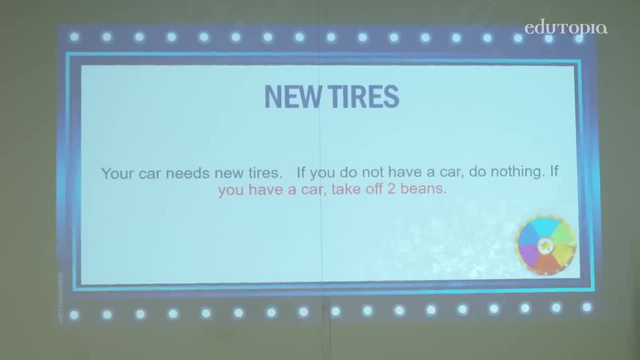 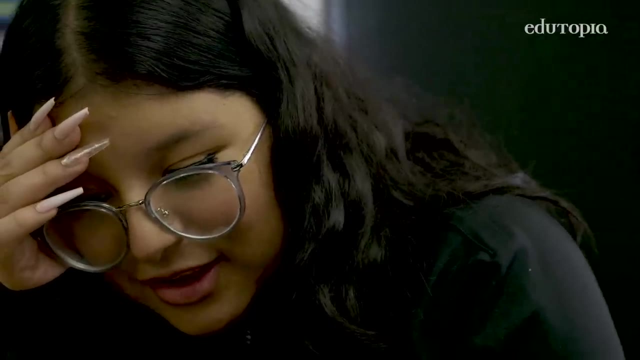 Stop, Stop, Stop. Your car needs new tires. If you do not have a car, you do nothing. I guess we're just going to have to go with no phone. No, but like we need a phone, Okay.